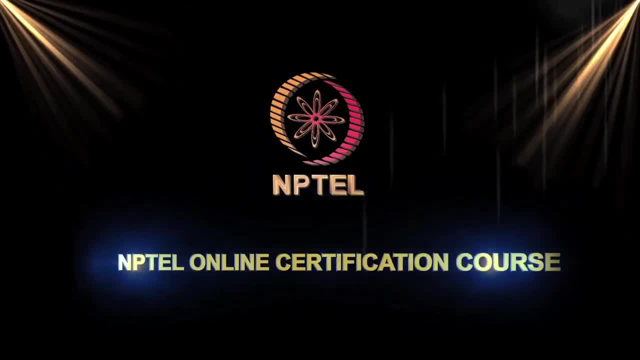 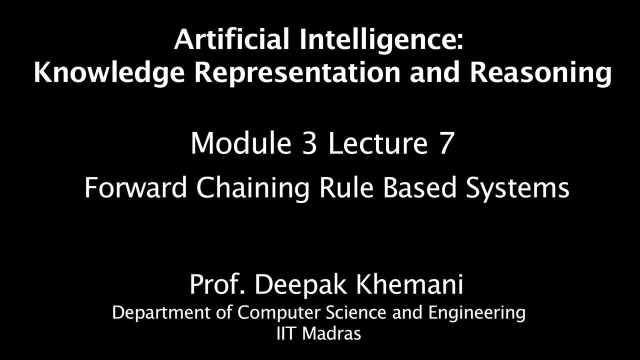 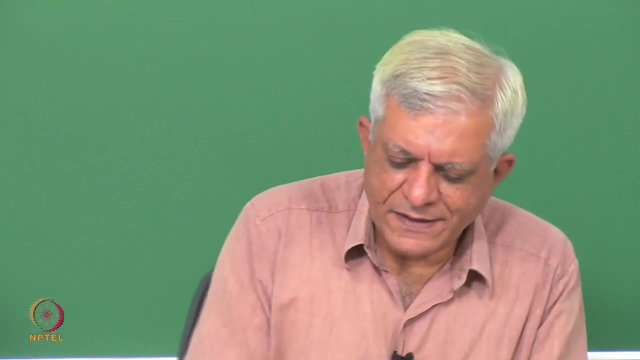 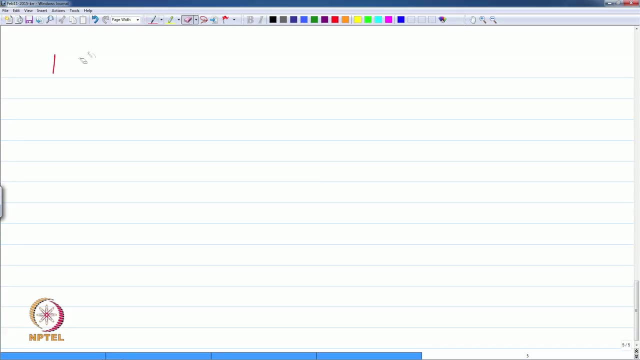 So in the last class we looked at unification. Today we want to look at power chaining again. So remember that we had looked at this rule called modified modus ponens, which was like modus ponens, So it uses unification because one may have variables inside the statements. essentially, 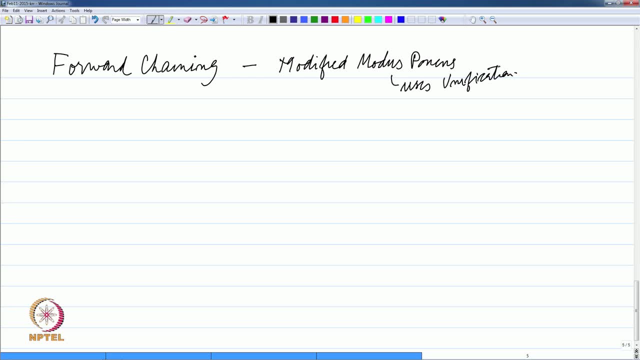 So unification is used to make them the same, and then you can use the modified modus ponens rule to apply essentially. So this modified modus ponens plus unification actually gives us a mechanism for able to reason. So now let us focus on the task of reasoning. 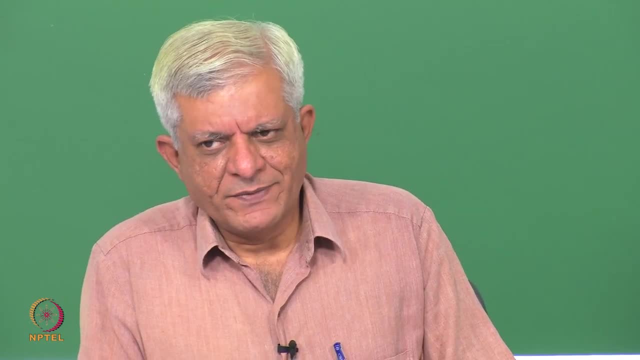 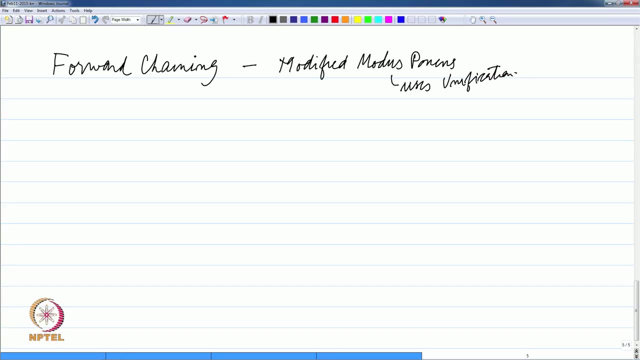 itself as to which inferences to make essentially. of the many possible inferences that you can make, which is the one that you want to make essentially Now? before we do that, I just want to make a comment that, as far as the knowledge representation path goes, the community which looks at these algorithms, or you might say 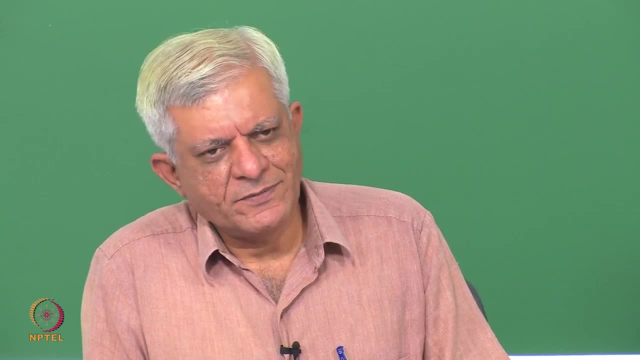 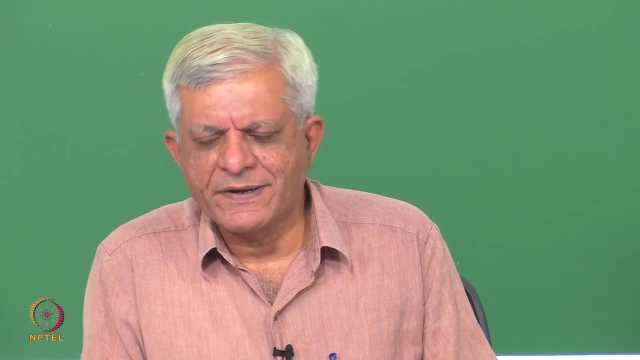 the mathematical inclined community or the logic community. they do not focus too much on how you are representing things essentially. So that is why we use variable names, like predicate names, like p, q, r. we do not particularly care what is the variable you are using. 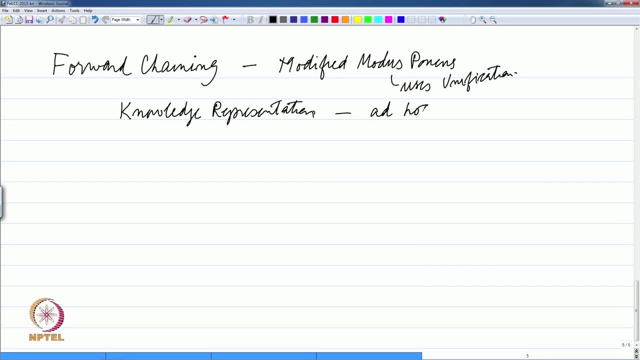 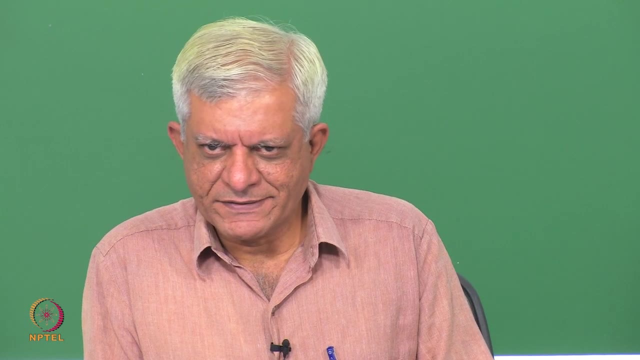 So in some sense, we are using ad hoc predicates. We are not giving any thought to the fact that whether these are the predicates which are the best ones to try to describe the domain that we are trying to describe, and so on- We will come back to knowledge representation at a later time- We want to focus now on the 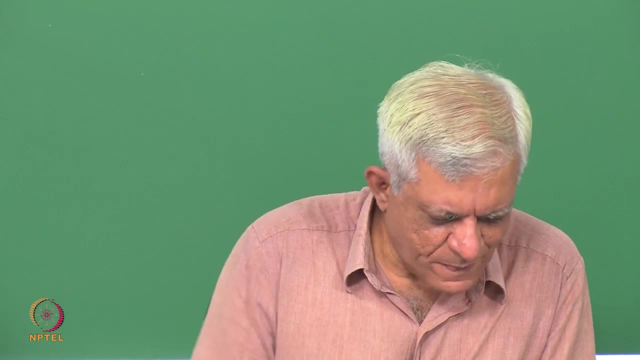 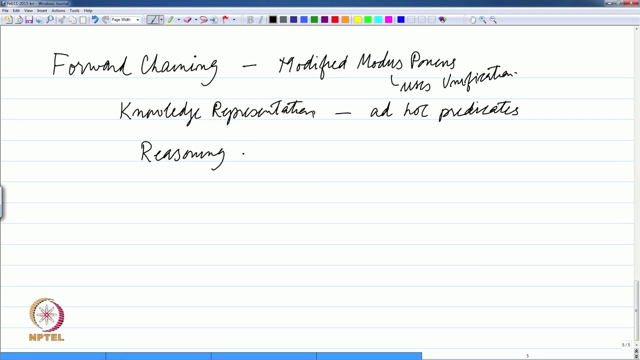 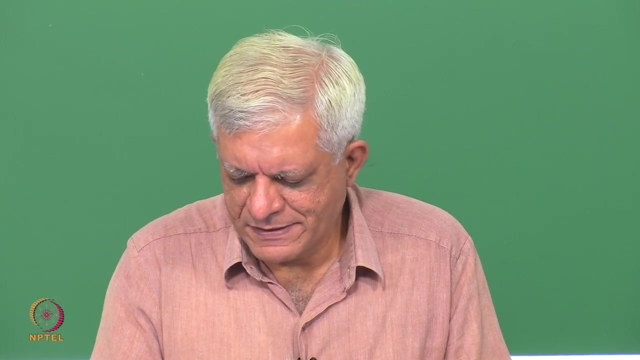 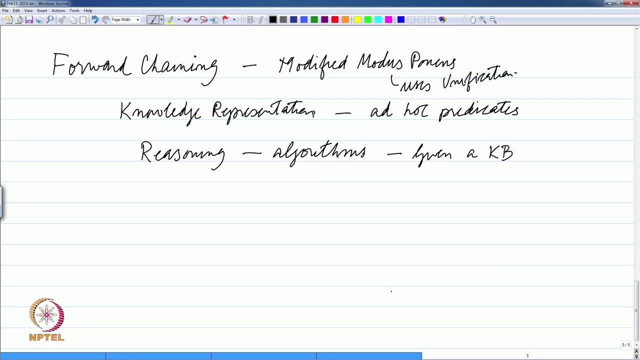 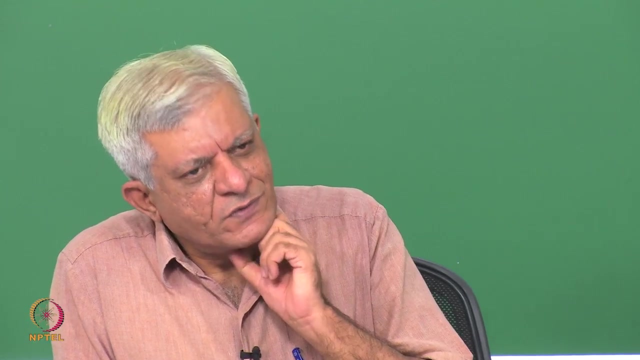 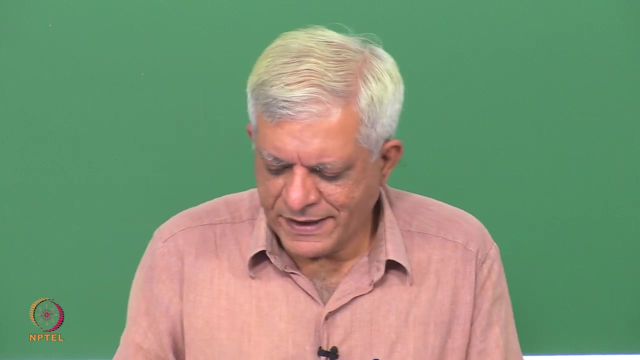 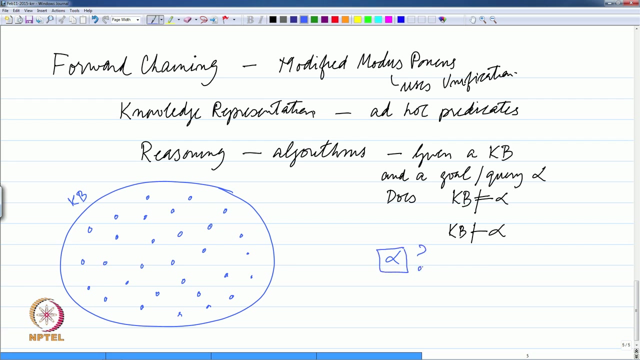 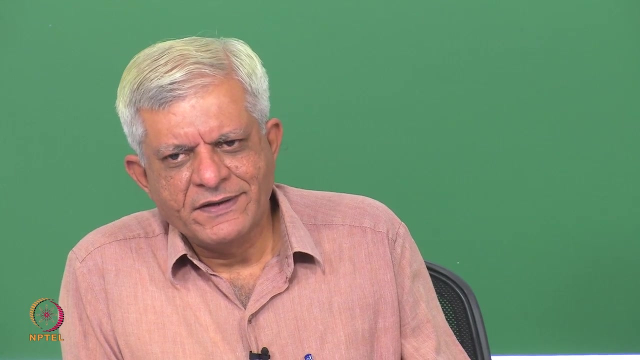 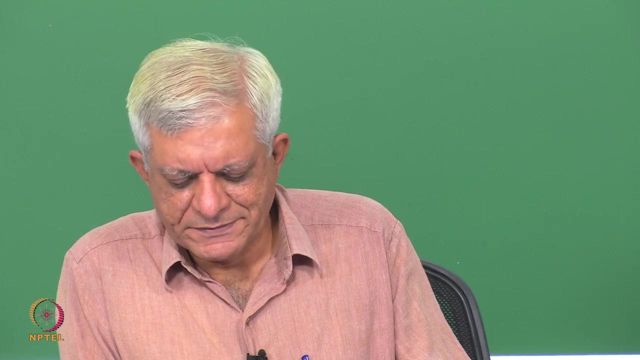 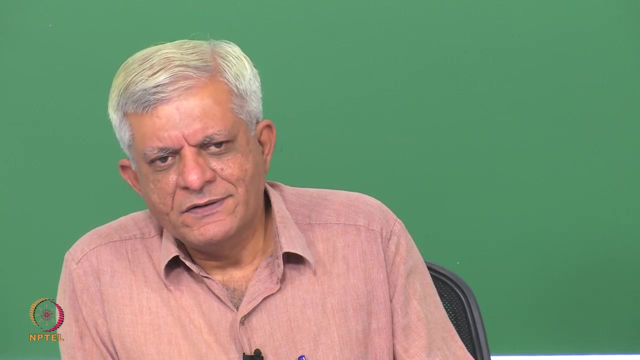 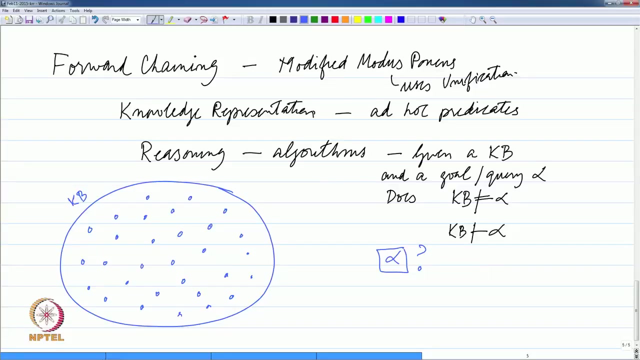 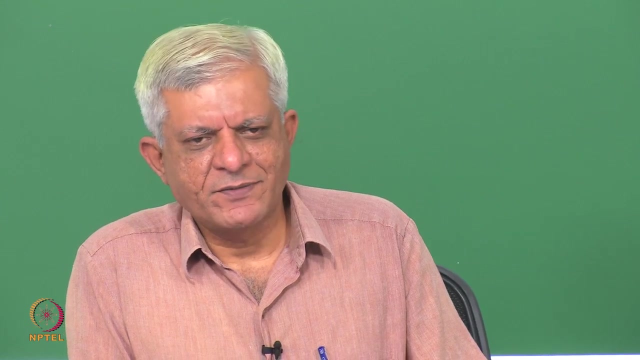 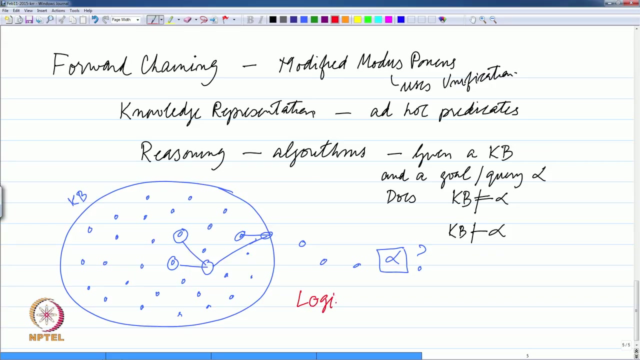 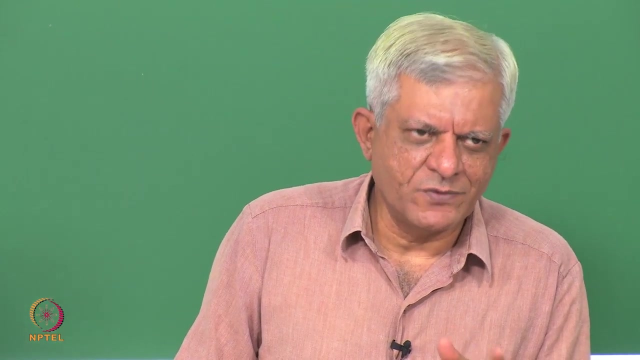 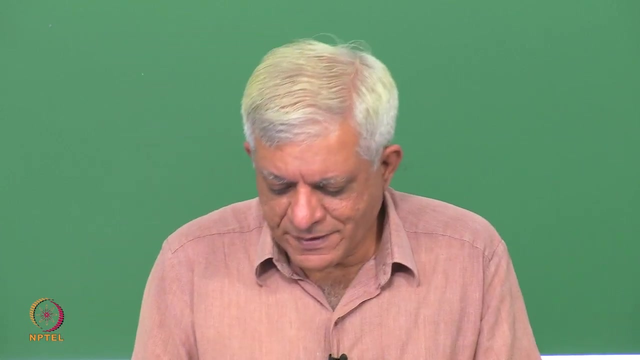 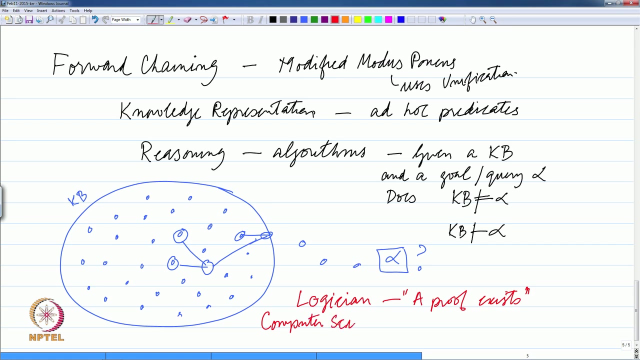 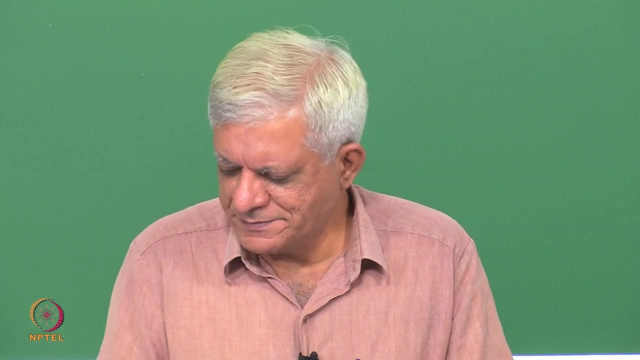 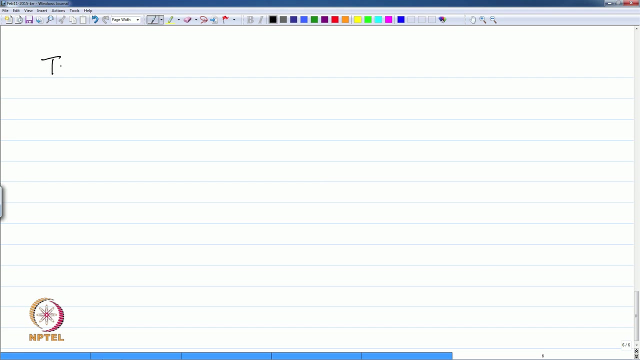 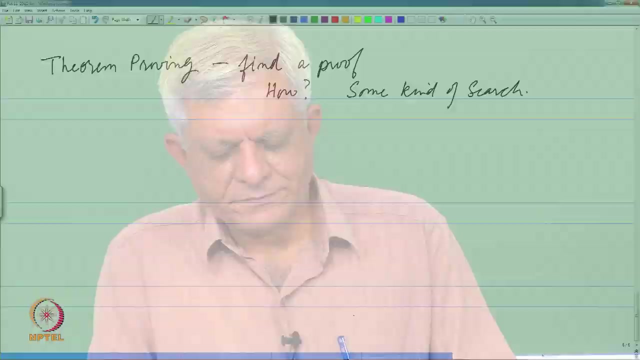 reasoning part essentially, which is the algorithms essentially. So the reasoning part is concerned with algorithms and we essentially want to focus on what is the algorithm that we want to use. So what we are going to consider to that is some kind of search, So as a high level, 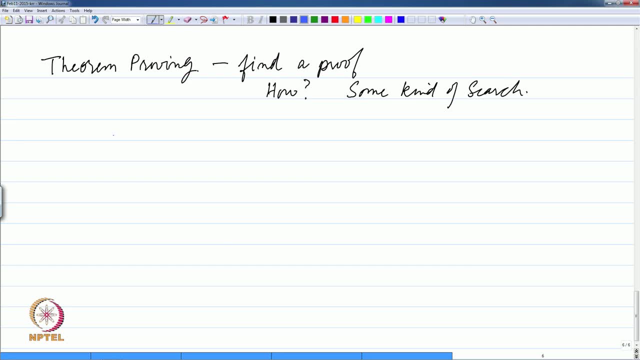 we have already said that the algorithm is as follows: Pick a rule with matching data. So we have already said that the algorithm is as follows: Pick a rule with matching data. So we have already said that the algorithm is as follows: Pick a rule with matching data. 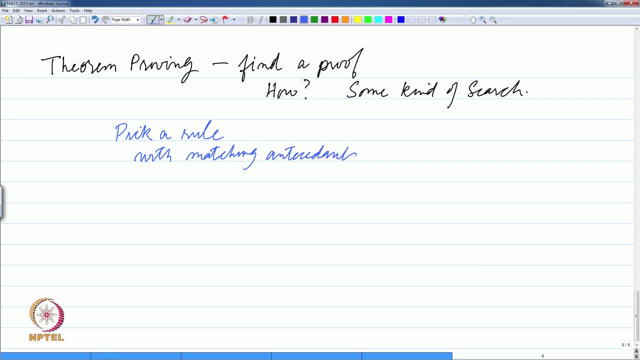 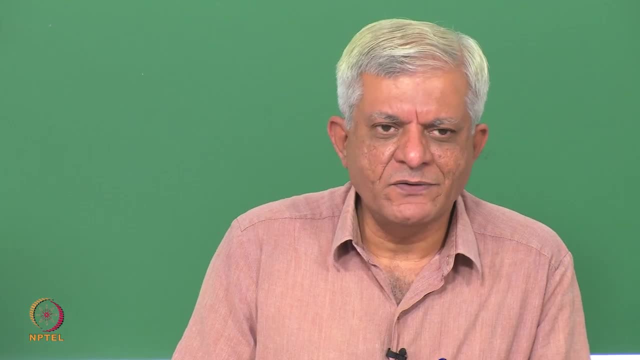 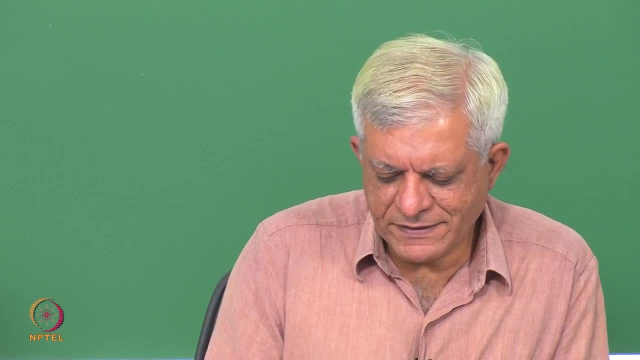 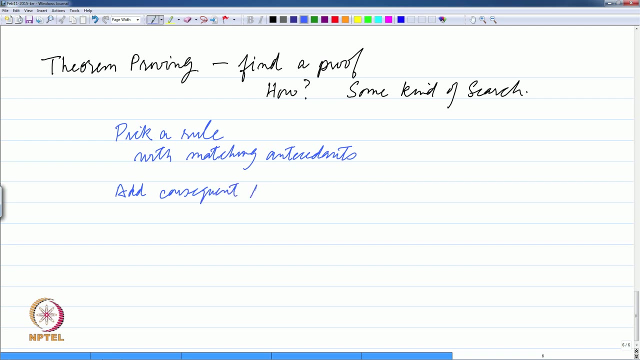 So we have already said that the algorithm is as follows: Pick a rule with matching data. So here we add consequence to the knowledge base. So antecedents are in the knowledge base. So in this way we keep adding more and more statements to our knowledge base. 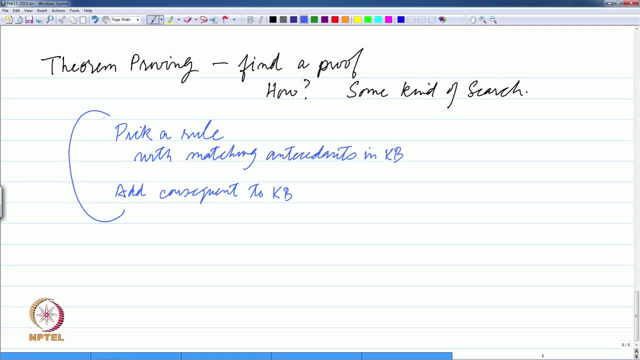 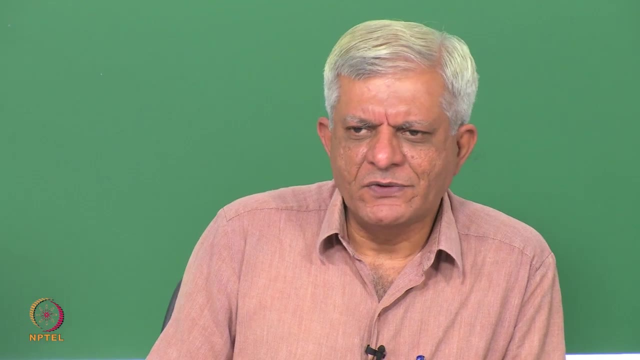 and we will terminate when we have added the statement that we are interested in the thing that we call alpha, essentially. So the question is: what kind of search can one employ? so what do we have? we have set of rules in this. we may have one or more rules. 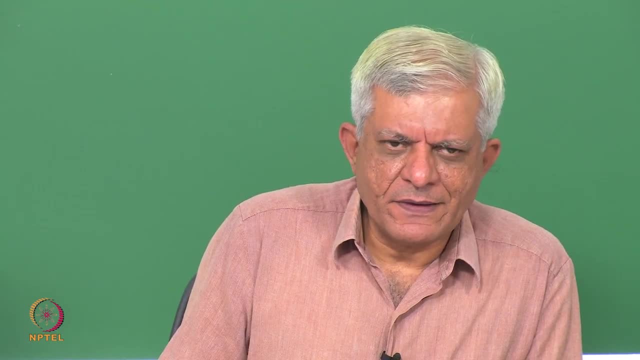 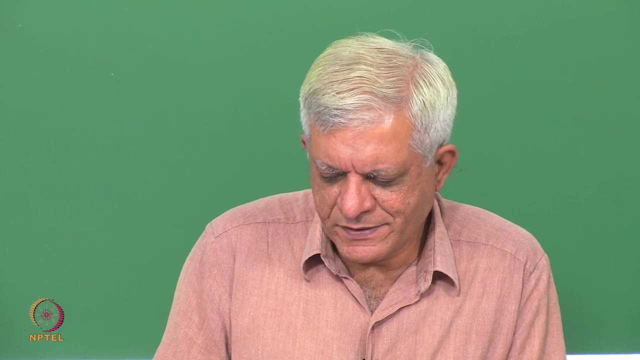 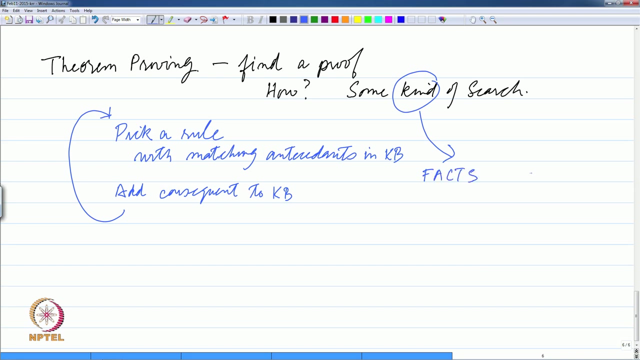 and we tend to distinguish between two kinds of things: one which we say are facts, and the other are rules. This is just a distinction that we use from the point of view of devising algorithms. both are statements in logic, but we distinguish between facts and rules. 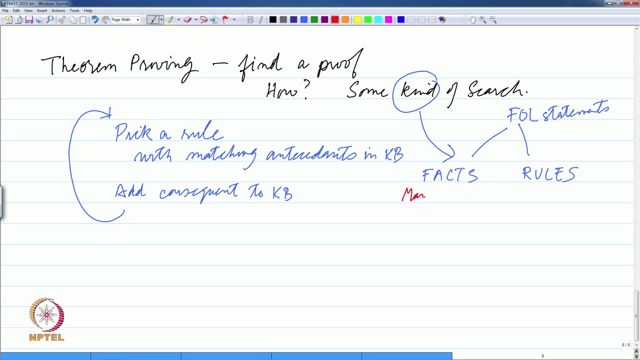 So fact, for example, may be man Socrates, and the rule may be for all x, x. So man x implies mortal. so I will just use m here or let me write so we distinguish between these two kind of rules. 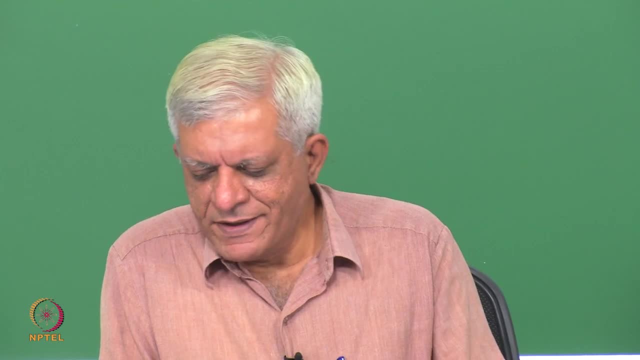 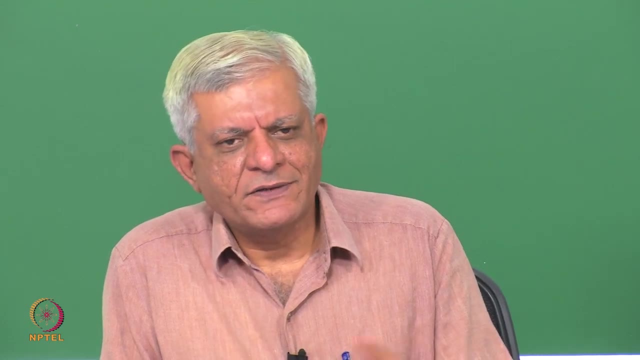 So, essentially, what modus for us, which is one rule of inference we are using, has access to a large collection of rules like things: all men are mortal, all students are bright, all bright students are girls, and things like that. whatever statements that we have, we 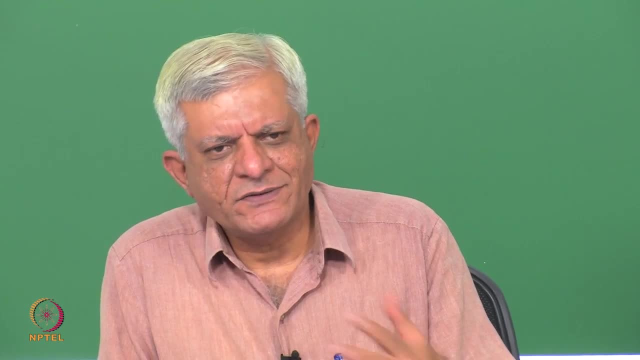 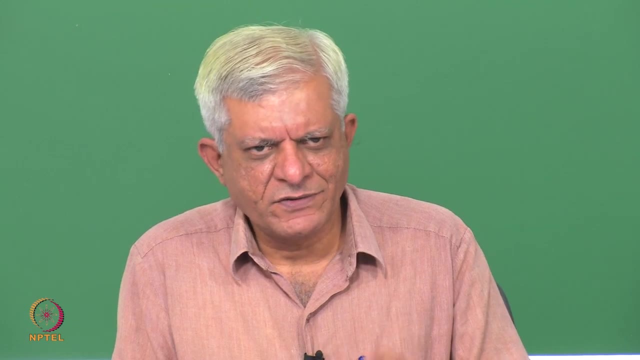 will call them, We will call them as rules and whatever facts we have is the actual data in the knowledge base, essentially that you know Socrates is a man and Shrestha is a student and Shrestha is a girl, and you know this kind of statements are facts essentially. 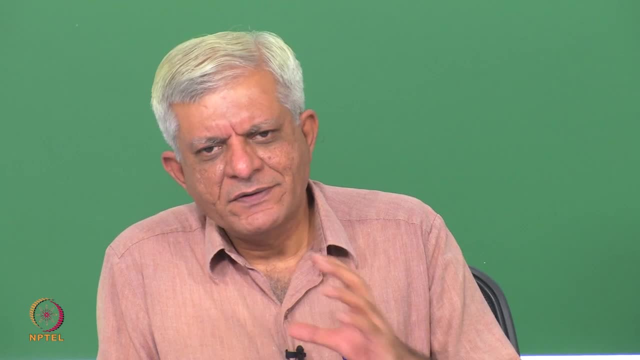 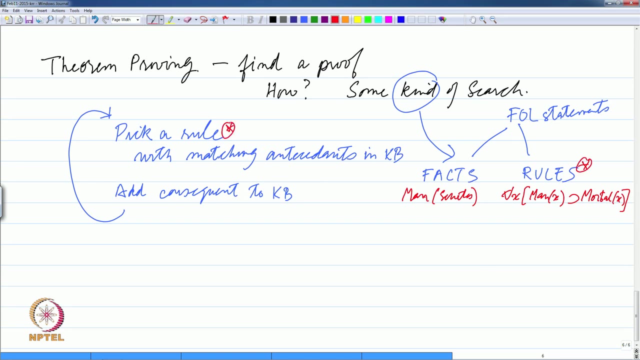 So modus ponens is trying to pick a rule essentially. so when we say rule here, we mean that is a statement that I mean here. these are also statements in first order logic. So there is a slight confusion between rule of inference and rule here. 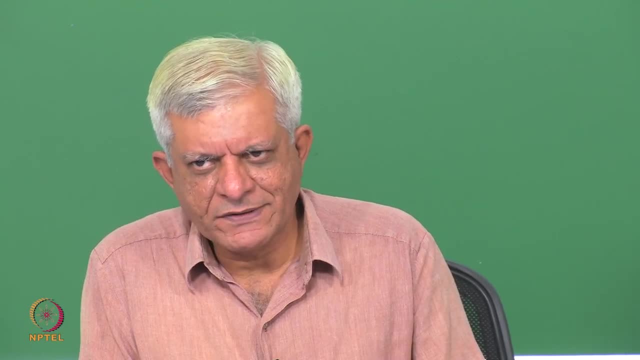 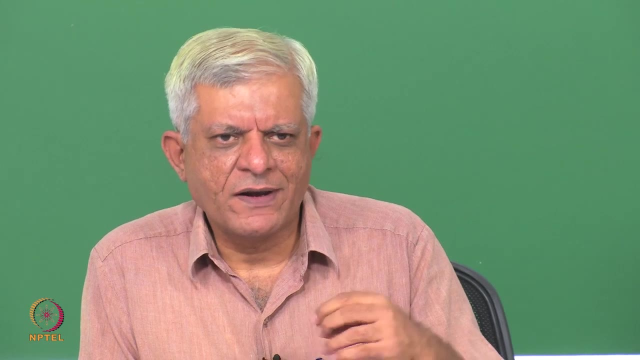 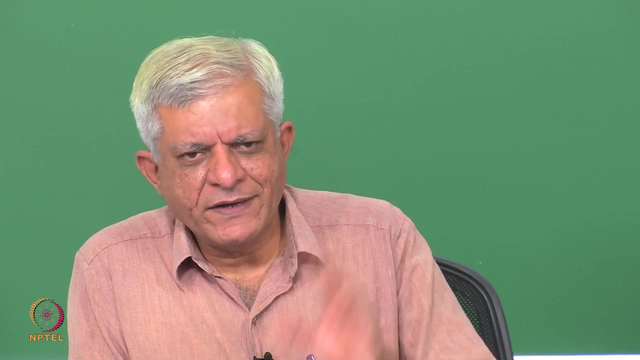 Rule. rule of inference is modus ponens or modified modus ponens. it is a meta level thing. Rule in the language is basically universal quantificates, statements, things like this: hat all x is, are, y is and things like that essentially. So the algorithm now needs weight through all the rules and all the facts to find something. 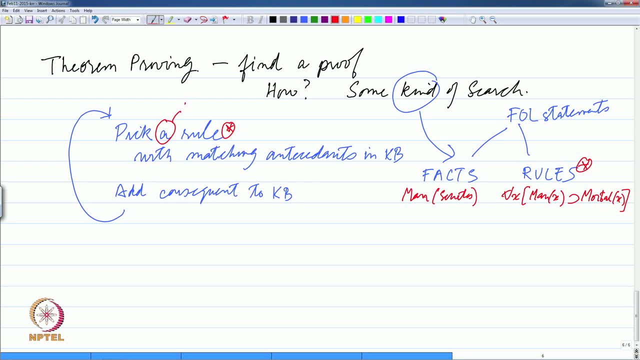 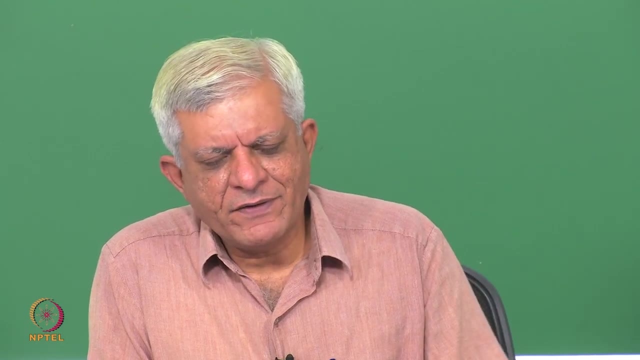 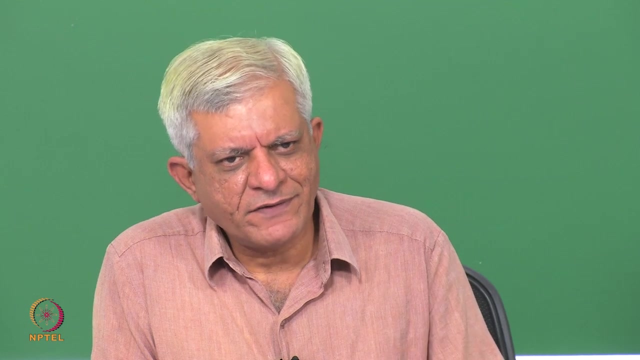 which is a matching piece of rule, a state, a statement which is a rule and a matching statement which is a fact. essentially Now you can see that if you have a large knowledge base, then the choices that you may have will be in proportion to the number of facts you have and the number of rules that 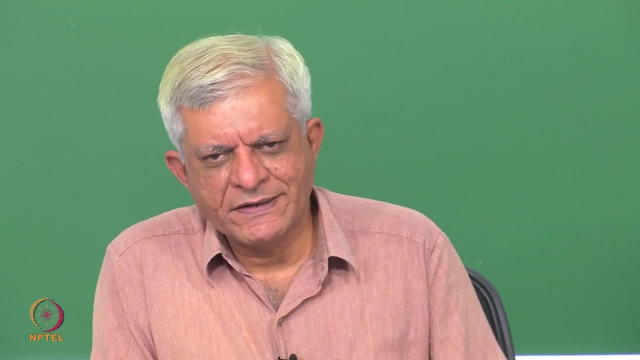 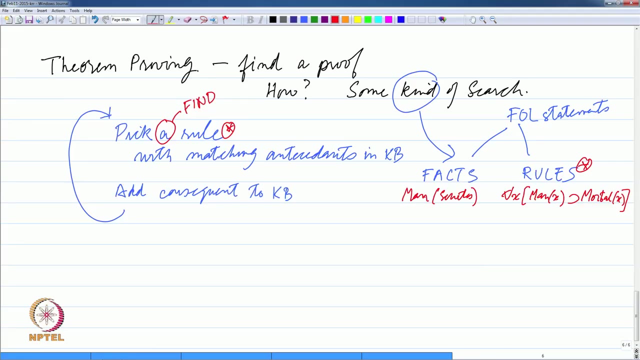 you have in your statement. So it is a. it is a problem which is going to increase comparatively in terms of complexity. So that is one of the main issues that we want to address essentially. So what are the kind of search algorithm that we can think of? 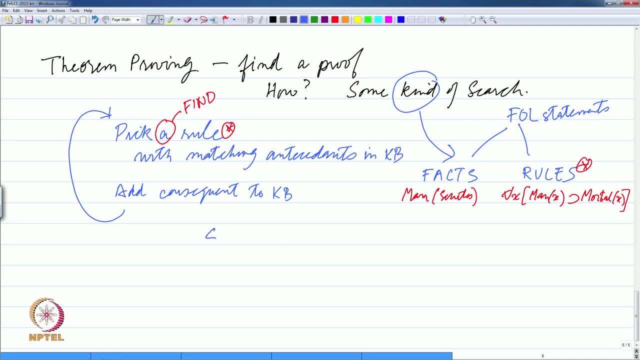 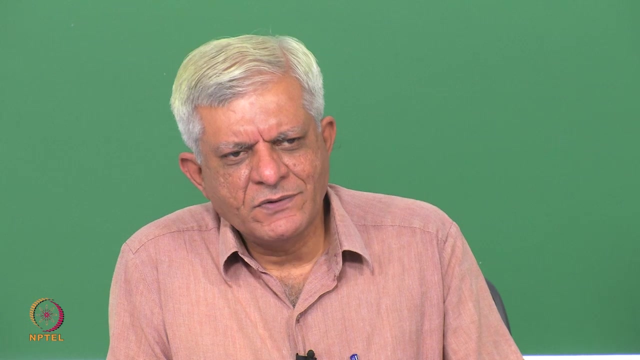 One is, of course, the simplest search is linear search. right is linear search Or sequential. this simply says: take the first rule, try to apply it to the first piece of data, try to match it with the second piece of data, and so on and so on. So you take: 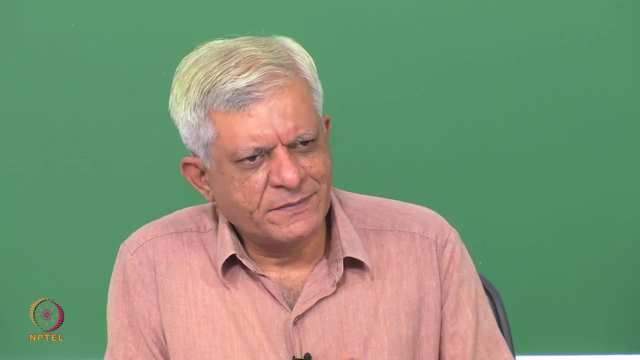 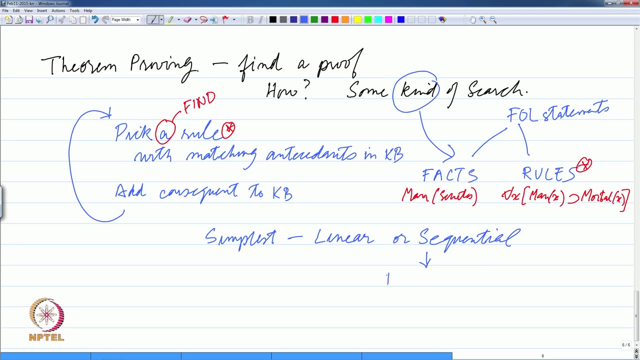 the rules one by one, then you match them with data one by one, and so on. you keep doing that. We will come to this later. essentially, This kind of an approach is actually used in a language prologue, And when we come to this, we will see that because we are using an algorithm which is sequential search- the 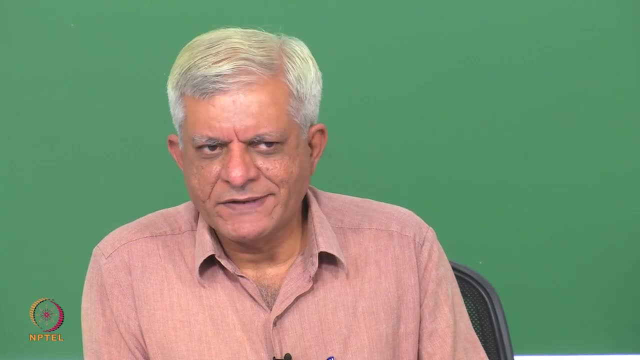 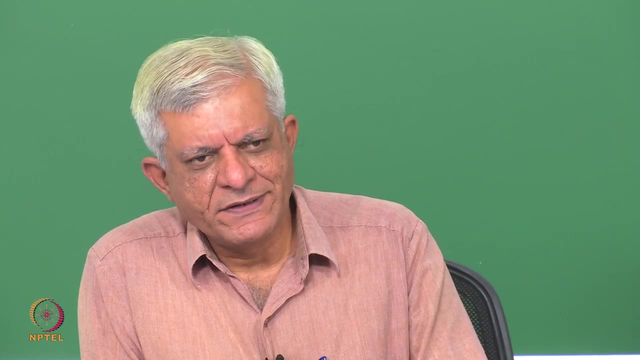 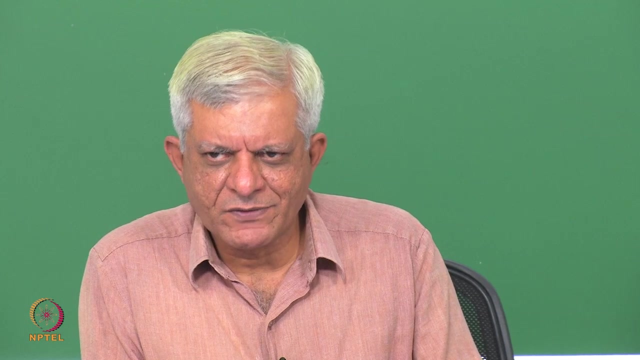 onus will be on the person who is writing the knowledge base or who is writing the rules, to put them in a certain order So that the algorithm will find the solution quickly. essentially, We will come to prologue, which is actually a process of backward chaining as opposed to forward chaining that we are looking at. 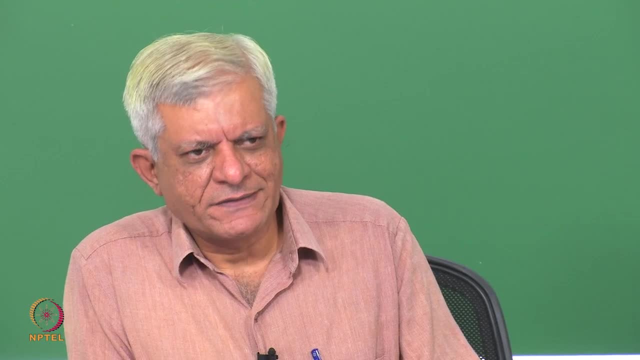 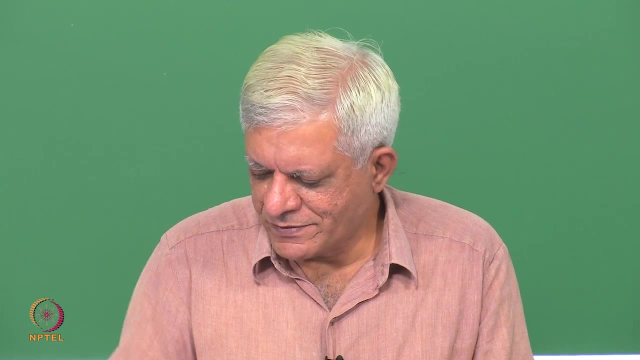 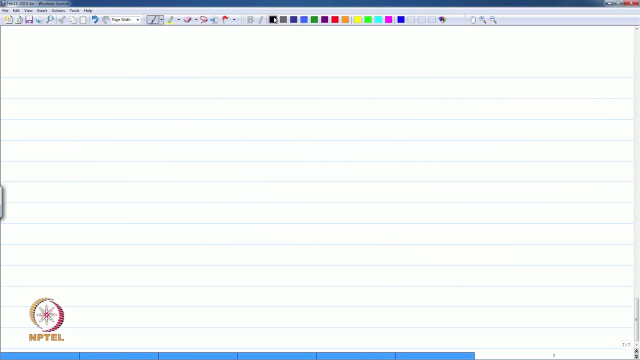 And prologue uses sequential search, So we will come to that little bit later. essentially So, today we want to see how forward chaining can be made more efficient. essentially So, we want to try to look at that aspect. 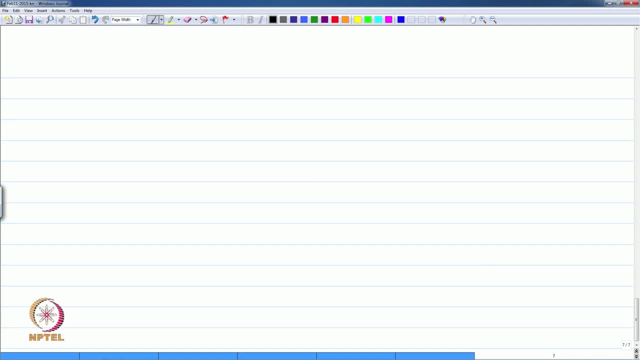 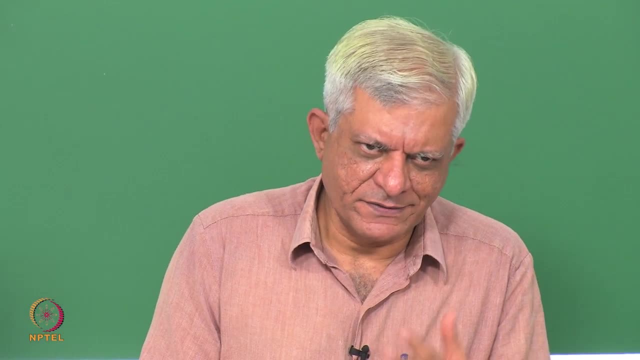 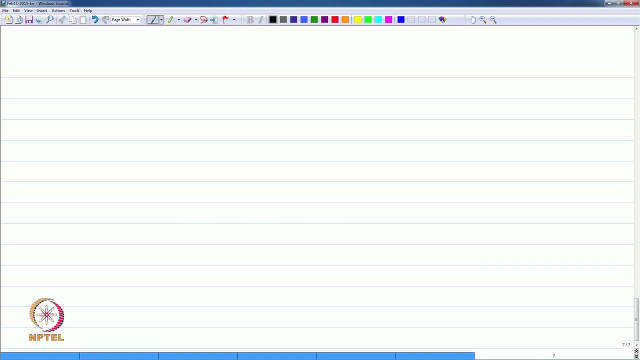 So what is forward chaining is doing is the process that we are saying: look for a rule, look for matching data, add the consequent and then keep doing that. essentially, Now, let us assume that rules are given to us in a particular format, which is So. when I say: 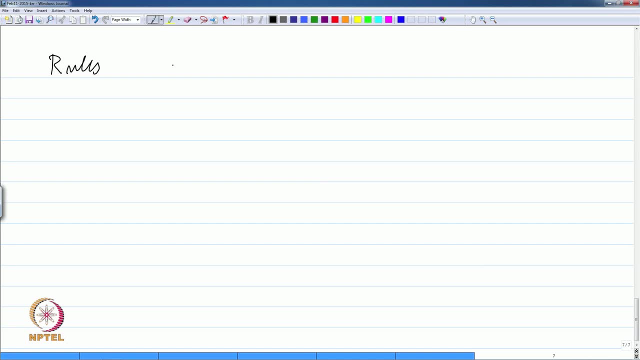 rules. I mean rules which are also statements in the language, or statements of the kind: if antecedent 1, antecedent 2,, let us say there are n conditions on the left hand side, then consequent, So we are given a collection. 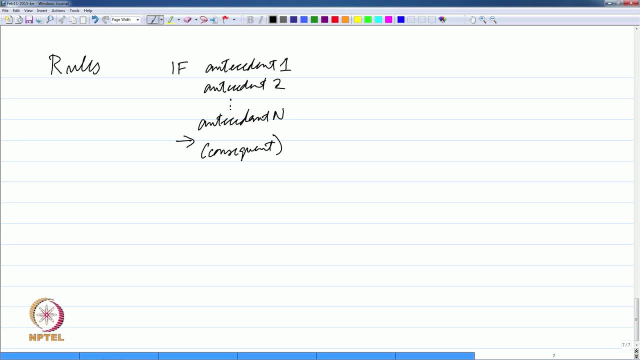 of such rules. So when you look at all these rules, we will have a set of patterns essentially. So these rules as such are the left hand side of the rules. We are trying to see where there is some element in the knowledge base which 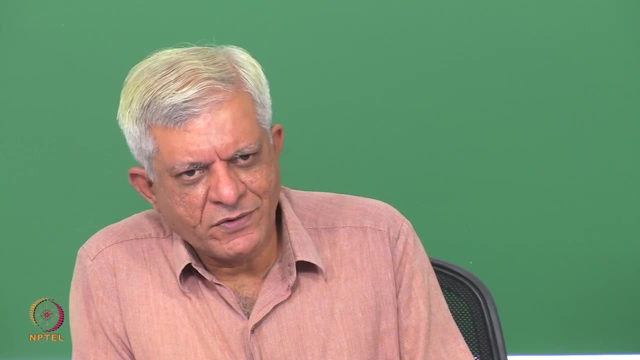 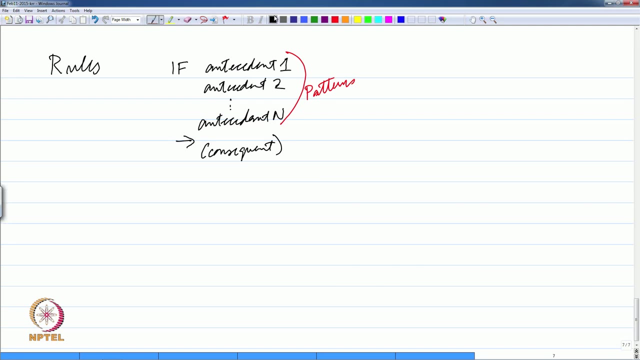 matches antecedent 1, some element which matches antecedent 2, and so on and so forth, essentially, And we are given a set of rules. So let us say that our knowledge base looks like this: I will have a set of rules for all the antecedents and that I am talking about. Then I will have 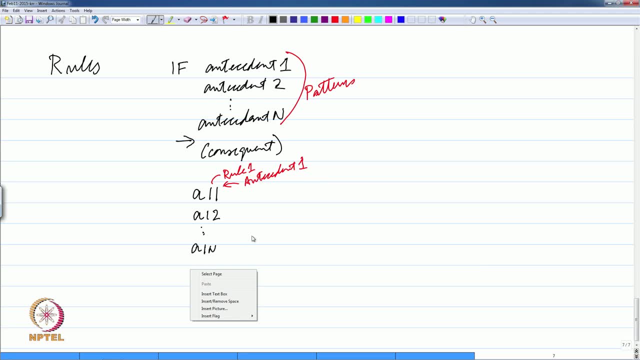 a 2, 1 and so on. a 2, R, let us say it has got R antecedents, and then so on and so forth. essentially, So for every rule I will have certain number of antecedents. So I will. 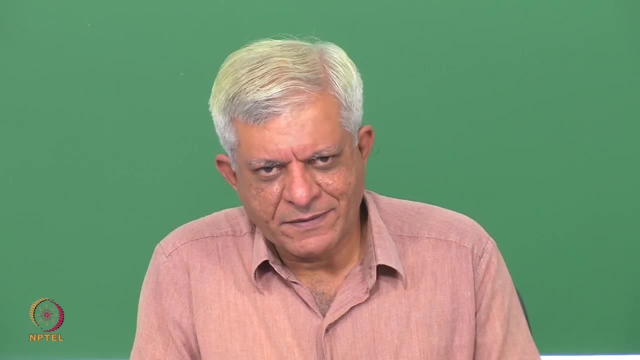 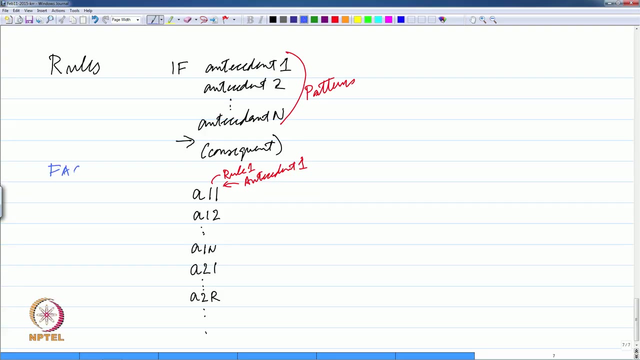 have a whole list of patterns that I am trying to match essentially. And what am I trying to match? match facts, right. So let us say simply: facts are some statements: data point 1, data point 2, data point 3, some number of data points we have essentially. 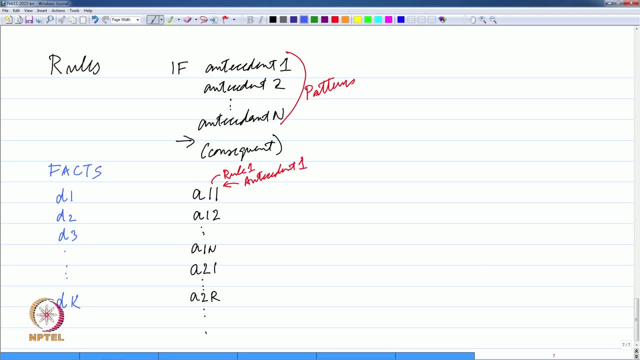 In the terminology that so that we will look at of our forward training algorithm that we will see, these facts are also called working memory elements And this of the facts are essentially called working memory And each of those data items is called a working memory element, essentially. 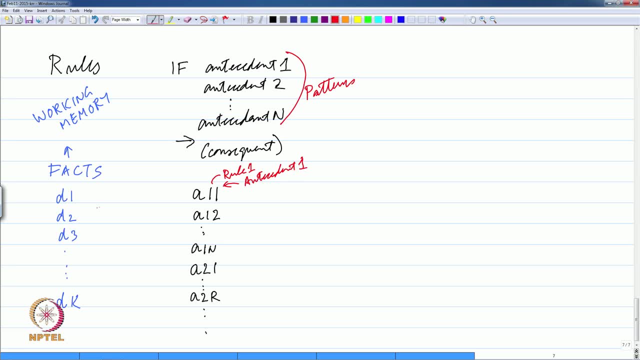 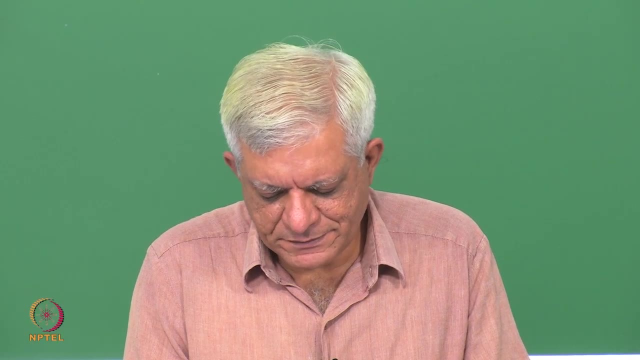 So what is the task? The task is you match a 1 with d 1, then you try match a 1 with d 2, match a 1 with d, and so on and so forth. So you can see that the total number of matches that we will have is that, if we have n, 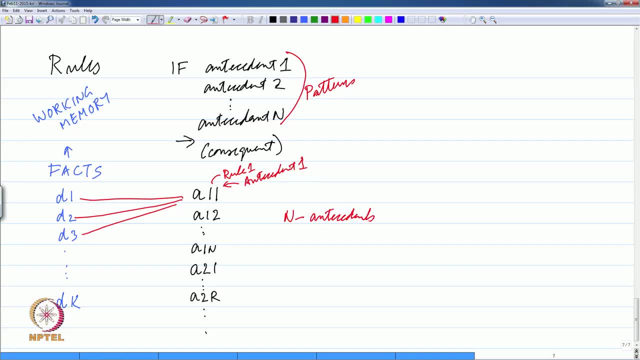 antecedents So n on the average per rules. if we have, let us say, r rules and d data elements, then we will end up matching every antecedent with every data element, essentially So n into r, into d matches. Ok, 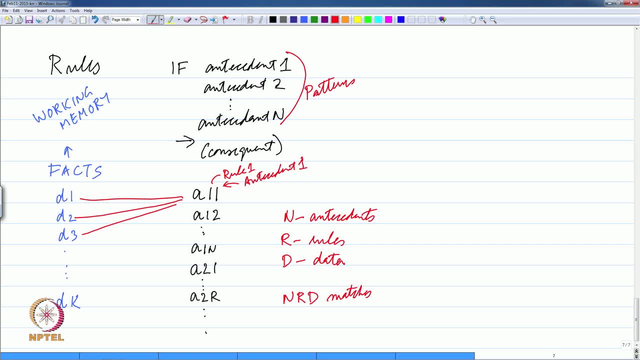 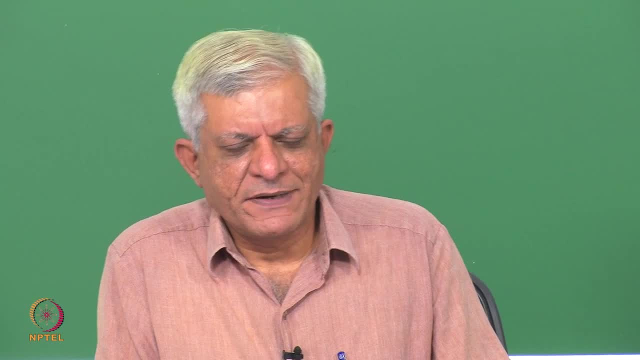 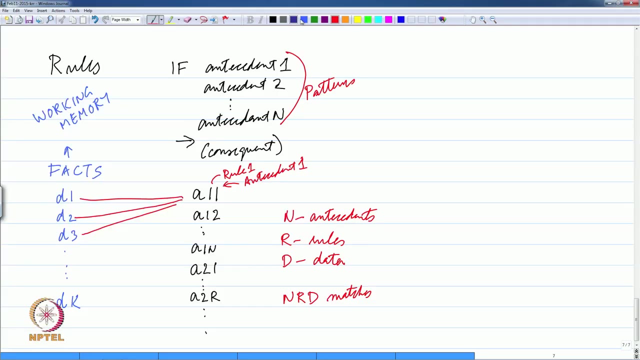 Ok, So this scenario is a little bit different from what I started by saying. I started by saying: pick a rule with matching data, but actually now I have moved to a slightly different way of doing things, which is the method that is used in what we call as production. 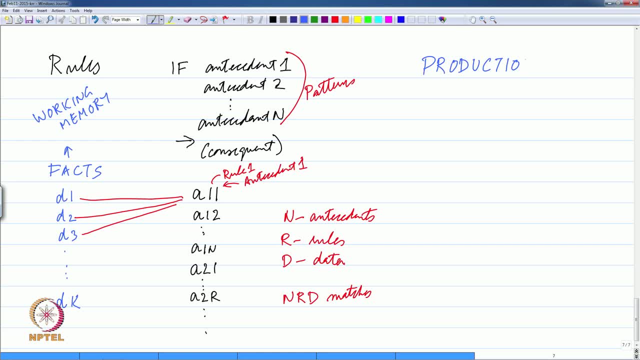 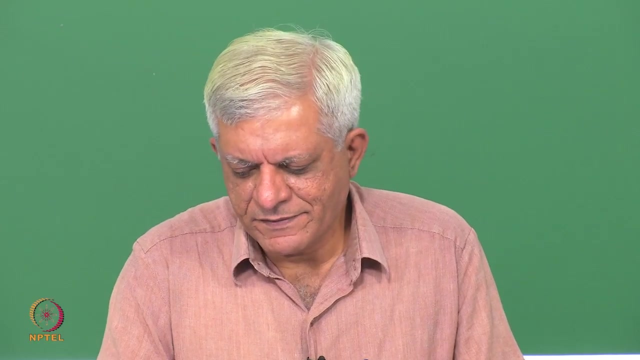 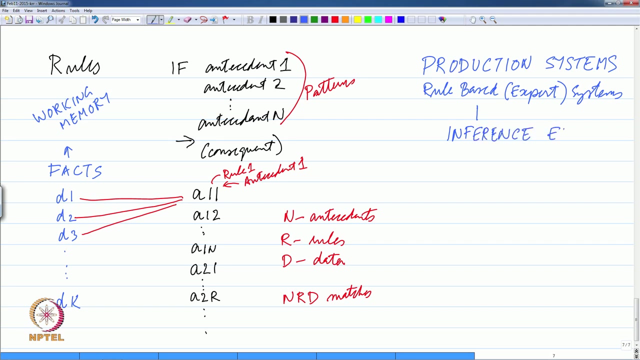 systems, Ok, a rule based systems. In the 1980s they would be called expert systems- And what a production system does is that it has something which is called an inference engine. Ok, Ok, Um. and one of these differences with inference engine is nothing but those chassis. 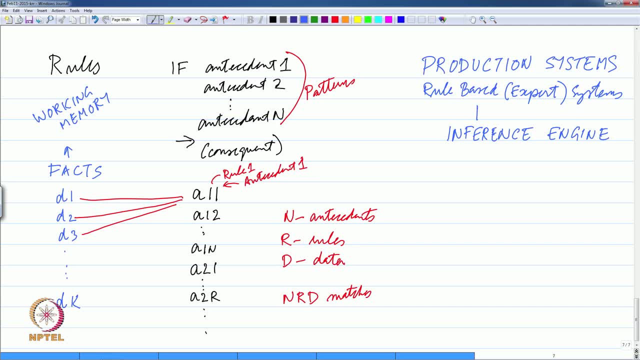 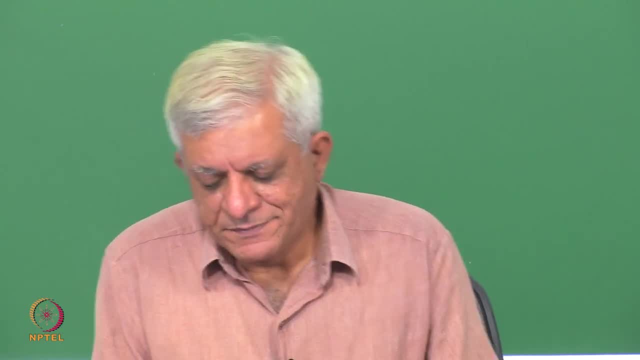 compression. this is terminology with these particular community uses. inference engine is simply the algorithm that we were talking about, which says that, you know, find I will with may add the consequency and so on and so forth, But the differences that the typical forward training, if is inference engineering, is made, 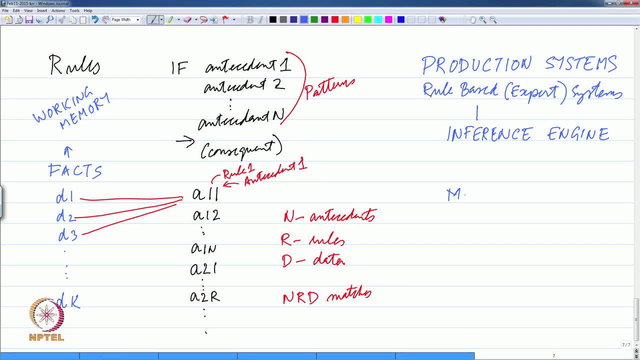 up of three steps There. first step is match, but- And the thing about this is the Yes pairs of the kind, some rule R i with matching data point. So d 1- 1, d 1 2, d 1 n, let us. 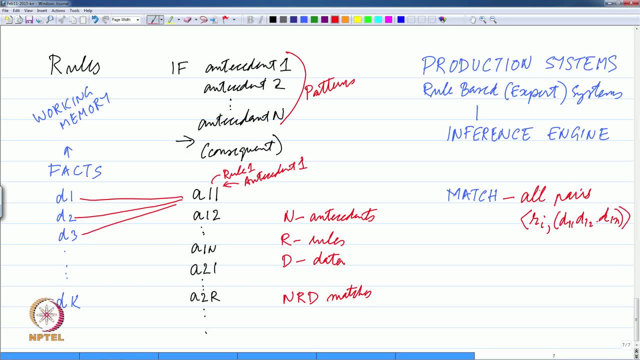 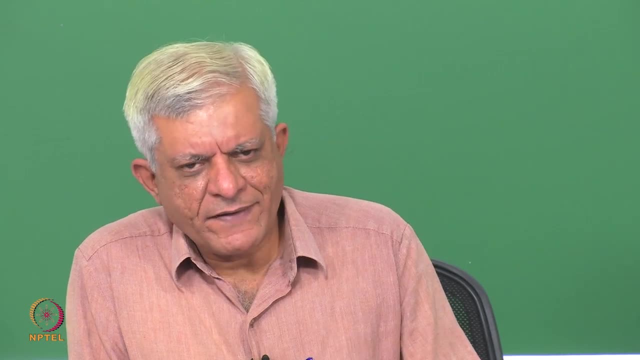 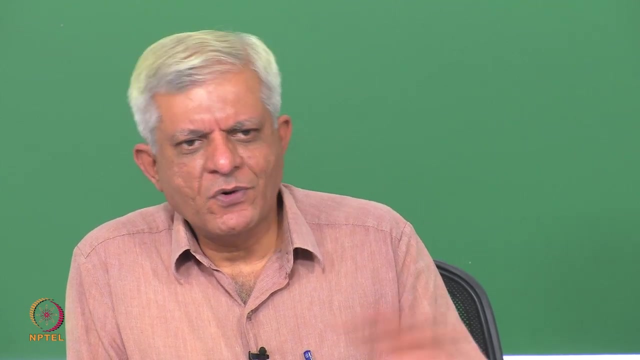 see find all such pairs. let me emphasize that. So the match part of the algorithm simply says: given a set of facts and given a set of rules- both are statements in first order logic- which rules are matching with which data? produce the whole set for me, and I will. 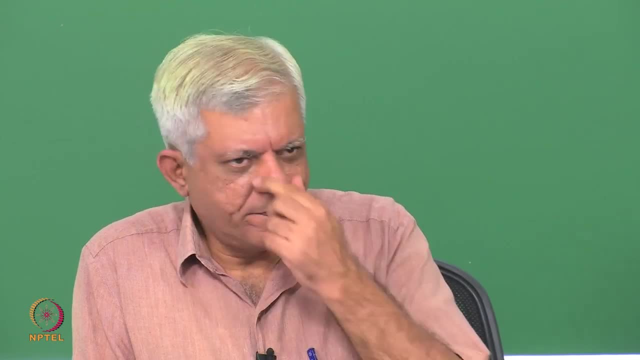 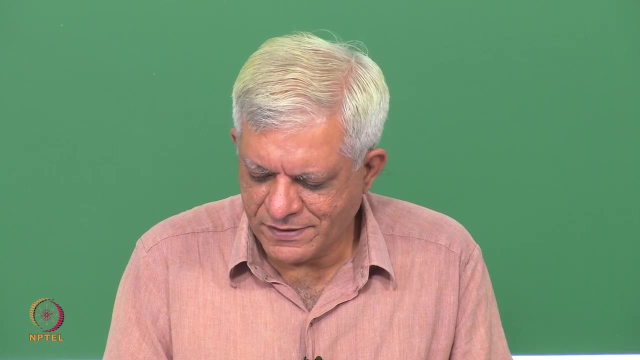 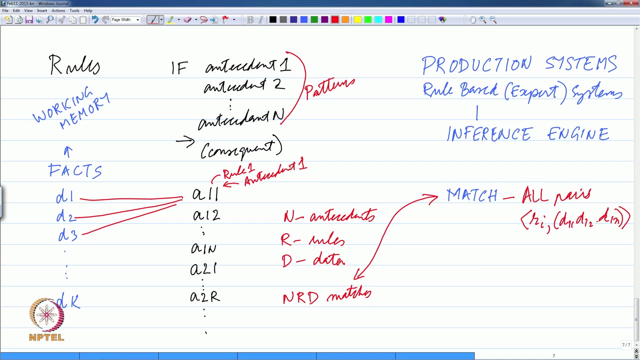 choose which one to select after that. So this is sort of doing a pre processing of match, essentially, and this match is what will do this n? r? d number of matches. essentially, Now that we have done all the matches, we have a step called resolve which essentially says: 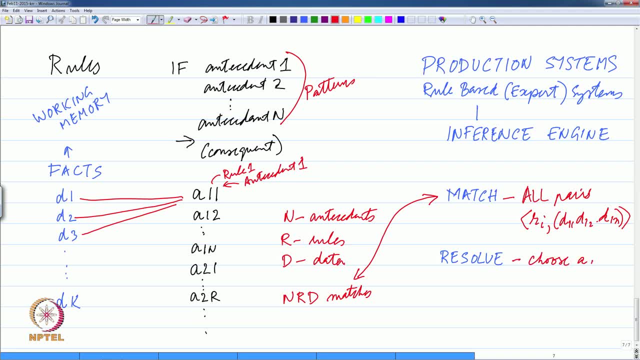 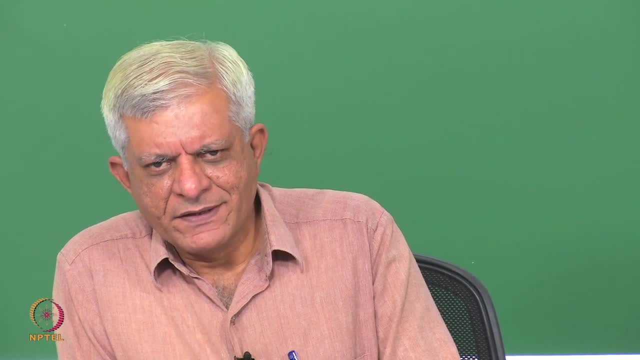 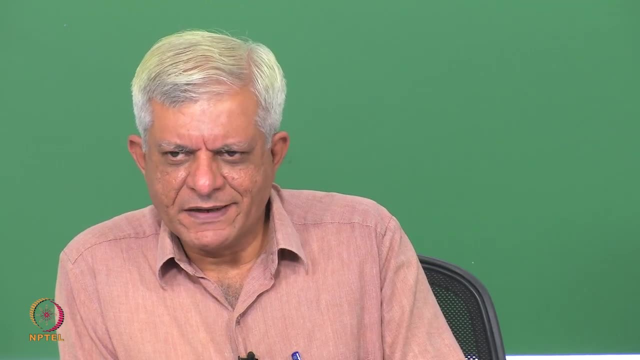 choose a pair. Obviously, it is very critical as to which one you are choosing. So, this element of resolution, how we? what is the problem solving strategy that you are trying to use? as to which rule you will apply? we will come to this a little bit later. So at the moment,